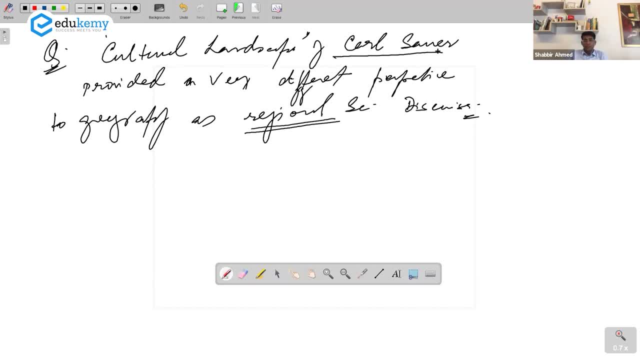 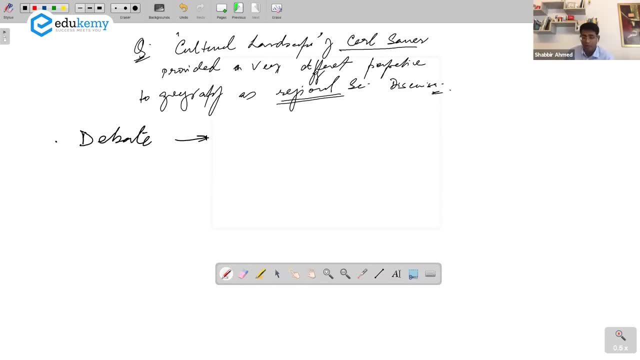 this a bit And it's a very integral part of regional science, very integral part of possibilism. So the debate has been on what is geography? So if I look at the perspective of Varanus, geography is general and special study of earth. If I look at Humboldt and 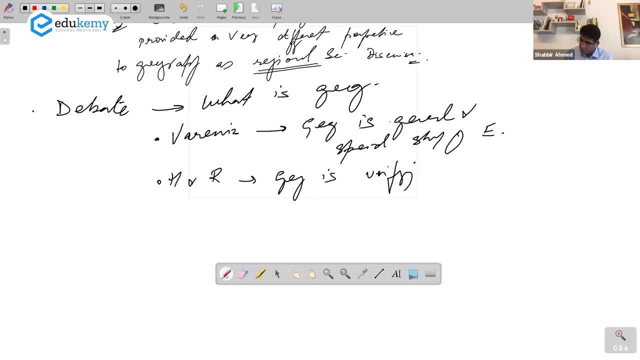 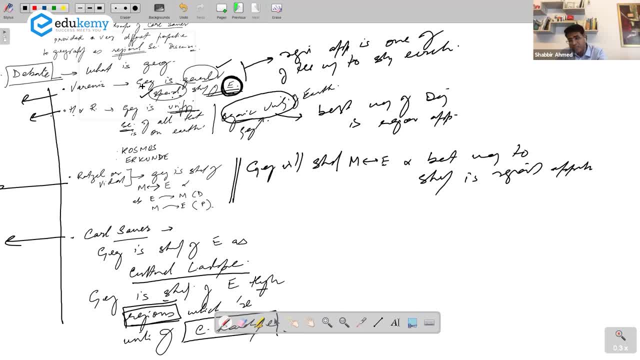 and Ritter. geography is unifying science of all that is on earth. So if I look at Humboldt ways of studying earth, which means regional approach, is not equal to geography. it is only one of the ways. Humboldt says that we will study organic unity and organic unity. 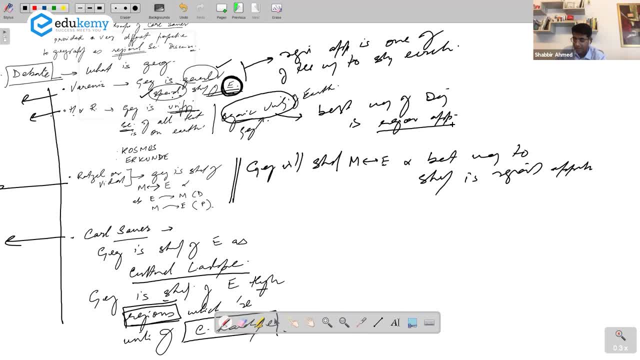 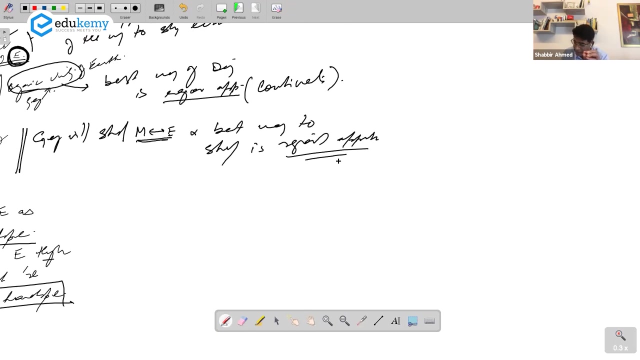 regional approach. the regions are at the scale of the continents: Africa region, Asia as region, Australia as region, and so on. whereas if you go to okay, they say that we are studying how man impacts environment, environments impact man. we think region approach is better in small, small scales. 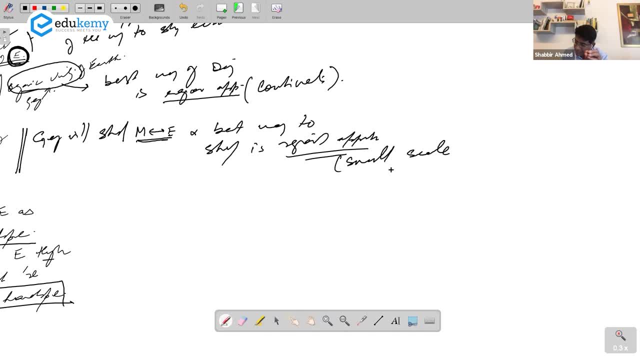 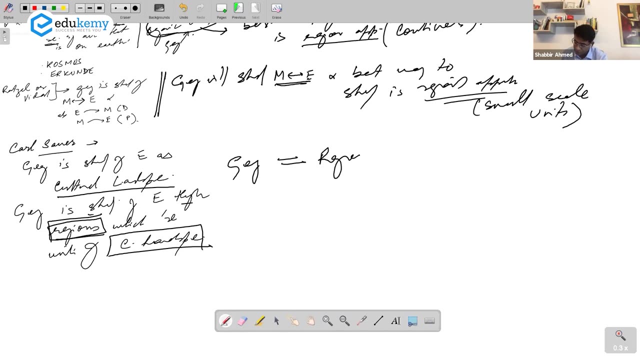 regions are small scale units, so region is a way of studying man environment relationship. is it okay? when you come to Carl Saar, he says geography is equal to the regional study of earth and the regions are the cultural landscapes. geography is regional study, geography objective. that's why. 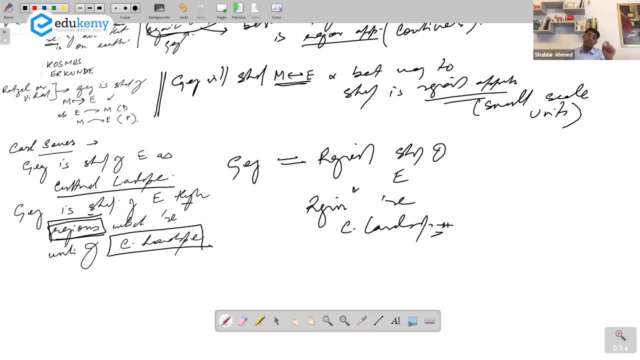 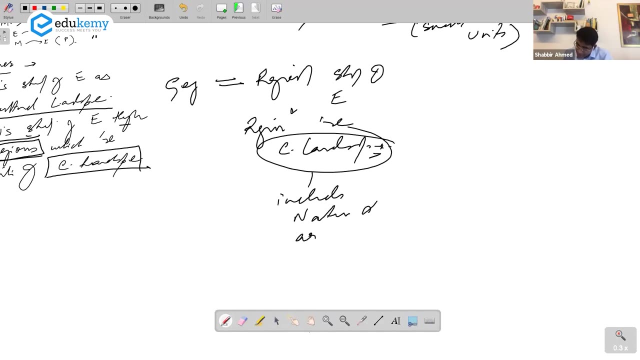 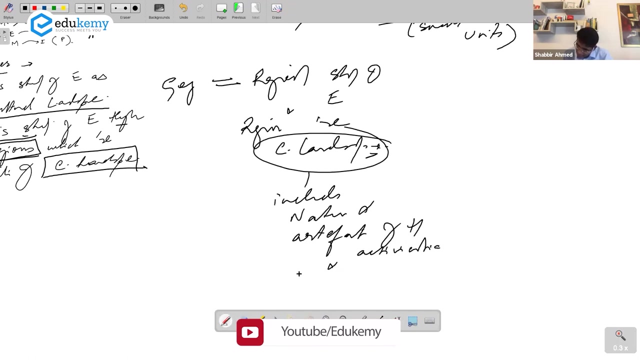 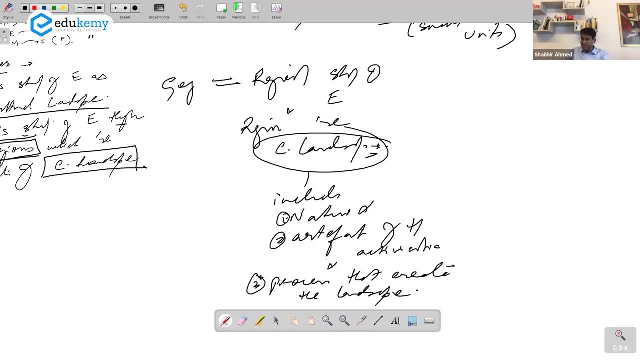 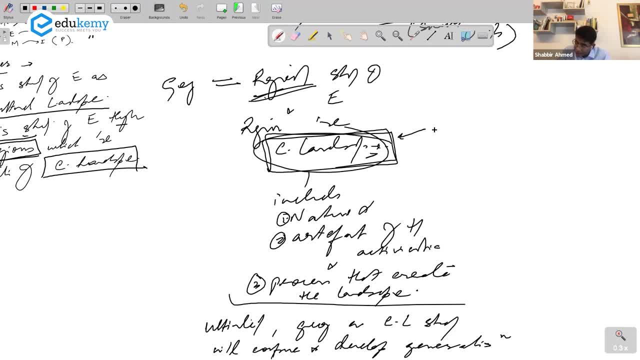 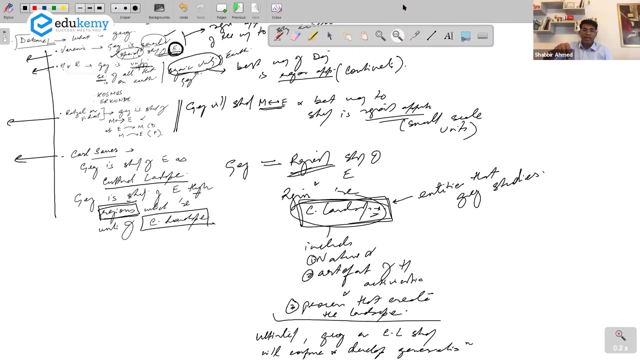 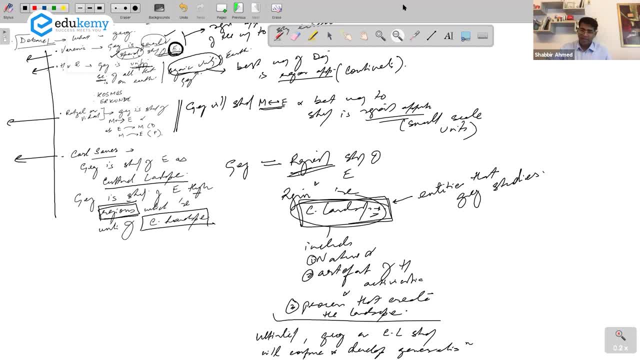 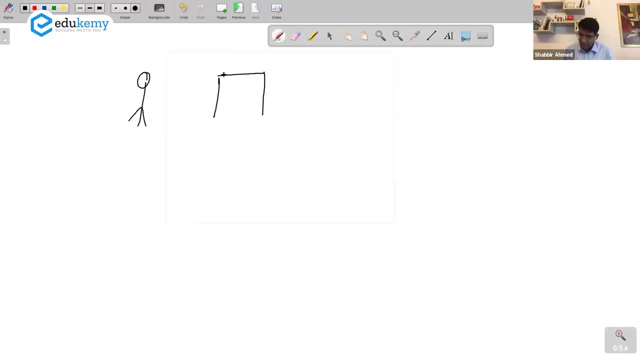 study is geography of a method. if i want to simplify, one last try. okay, one last try is example. there is a man, he lives in a house. one man says: i will study the man and for knowing him better i will also study his house. other guy says: i want to study the house. 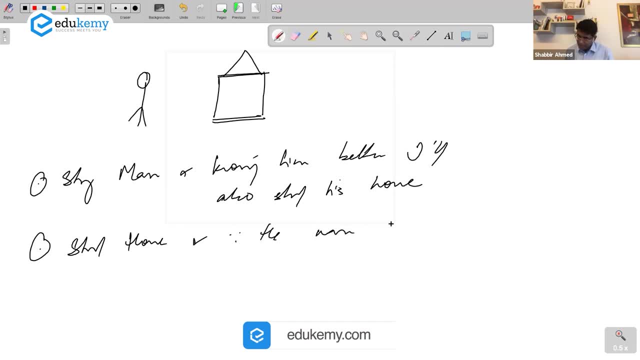 and because the man lives in it, i will study him. to study of man is the object. studying the house is one of the ways of doing it. other guy says no, because man lives in it, i will study the man too. which one do you think is razzle and which? 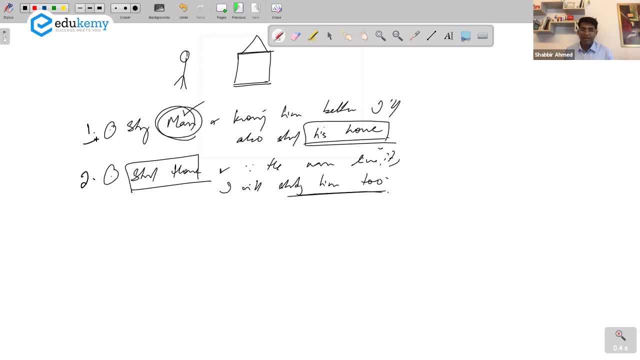 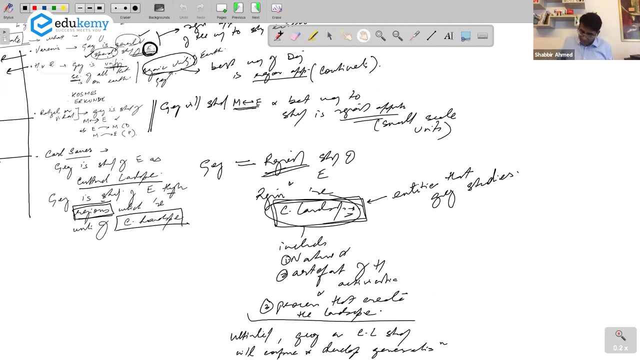 one. do you think is is Kalsor. If you understand this, my work is done. Who is Radzil and Vidal in this? Who is Kalsor in this? This is Kalsor and this is Radzil and Vidal. So, anyways, have you understood now What is Kalsor saying? What are these details? If you understand this, then you have got no issues. Let's go back now. What is Kalsor telling us? 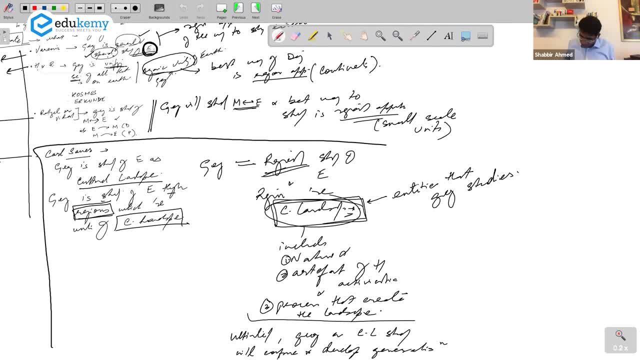 Geography is regional. geography is what Kalsor is talking about. The geography is equal to regional study And the region's name is cultural landscape. We study the nature, We study artifacts. Artifacts means whatever is part of the human creation. And third is the process that creates the landscape. 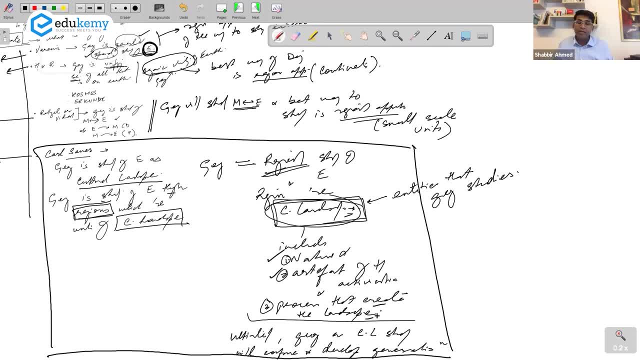 The entire process. What is that? Where the landscape is created? The process includes history, The process includes cultural events, The process includes what we do with our nature And, ultimately, all of this for what? For comparing and developing generalizations about the earth. 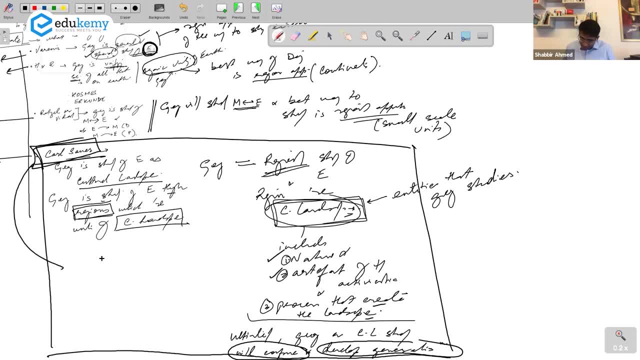 And this version, this Kalsor's idea, is very similar to Rich Tofan's idea. So Kapi is one of the first authors to research the geography of Kalsor. So Kalsor is in many ways the true regional approach in geography. 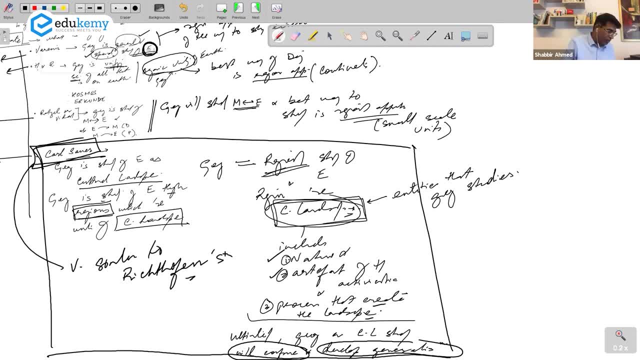 So now I would like you to open up the page so that I can explain things to you. now, Page 117.. So read with me. Look at the fourth line. it says By the beginning of 1929, 1929 is important. Why? Because 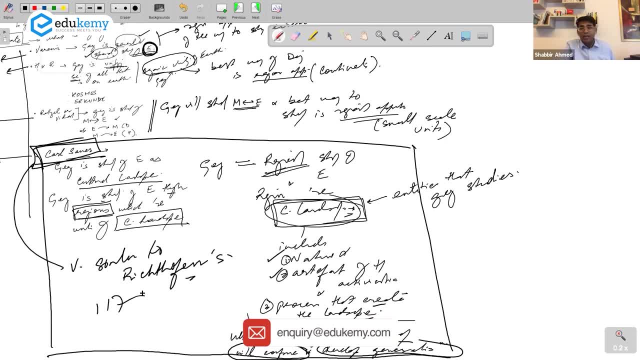 Possibilism of Vidal has got established, The principles of human geography, Okay. Okay. ideas of possibilism was established, okay, with this book. so by now we know possibilism is a school of thought. so it says: by the beginning of 1920s, many among the young generation of 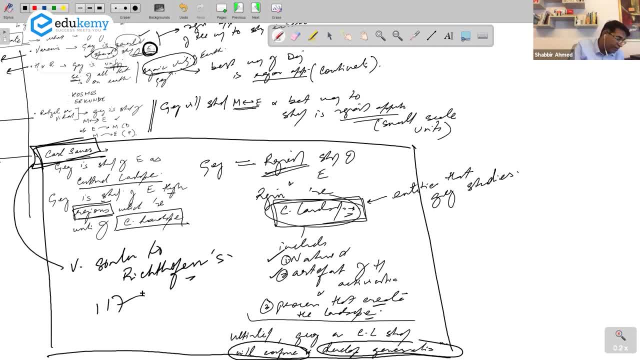 geographers had started the question: the validity of the content and method of geography as discipline built around man environment relationship. who is talking about man environment relationship? yes, radzel and vidal. so now questions are now being raised. is this what geography is? should geography study man environment relationship the new generations of students? 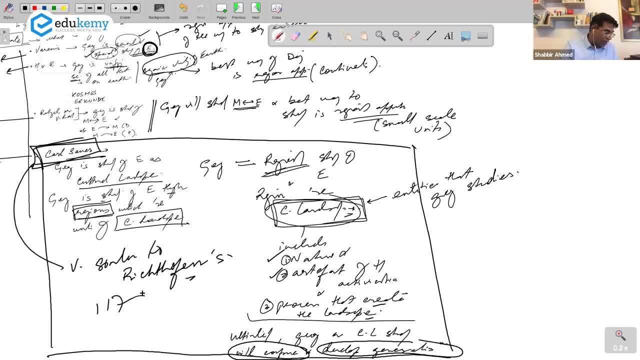 was anxiously looking at an alternative model of geographical work to replace the existing one, which they were finding increasingly unsatisfying. now next section: deko sor proposed an alternative model for geography in line with the humboldt and hettner saw, defined geography as a study of things associated in area of earth. 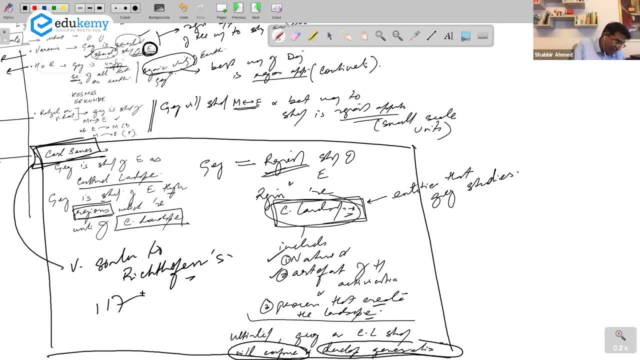 surface and the differences in nature of aerial aggregations from place to place, with regard to both physical as well as cultural factors. so what will geography study? geography is a study of things associated in an area. we take up an area and we study everything that is associated with. 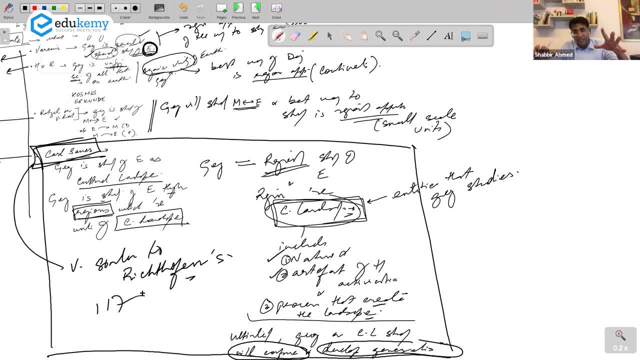 each other in that area. my study is the house and inside the house i study everything that is part of the house. so, rather than studying man, environment relationship and seeing a regional approach as a method, now we are studying that geography is a region study and inside the region will study. 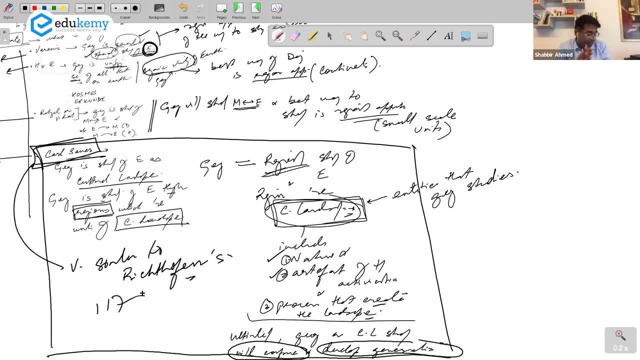 everything that are associated with one another. okay, in particular, he drew attention to geography. he drew attention to the role played by human action in modifying the physical and the biopic features, and so on. so look at the last two lines of the page for carl sauer: geography. 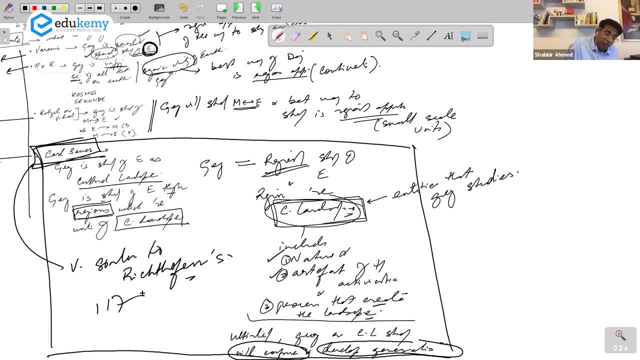 was the study of areas. for carl sauer, geography was study of areas, but not as description of areas as unique occurrence. so carl sauer's approach is not aerial differentiation. the objective of carl sauer is not to describe why the region is unique. 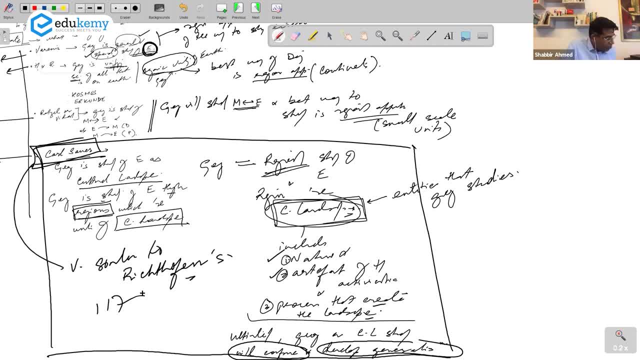 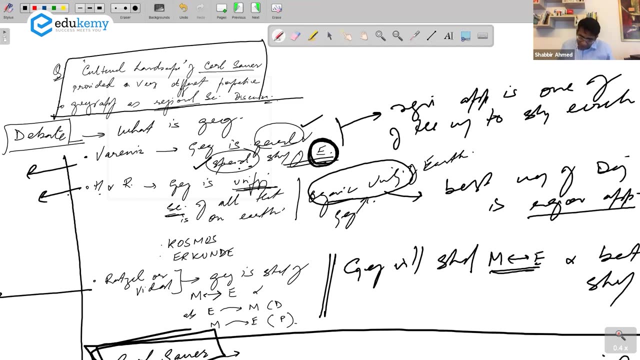 the purpose was to identify regularities and occurrences, to provide material for formulating generalizations, okay, and so on, study processes and so on. so now, if i go back here, what was the question? like carl sauer, provided a very different perspective of geography as a regional science. 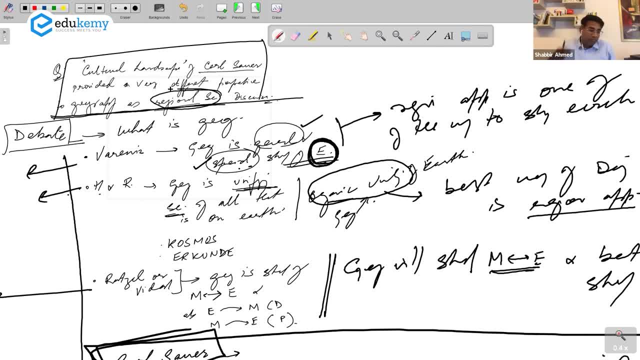 so it is different from the region of varanus, different from the regions of humboldt and vidal, different from the regions of radzill, different from the regions of aerial differentiation. discuss. so, if i write, this cultural landscape of carl sauer provided a very different perspective.